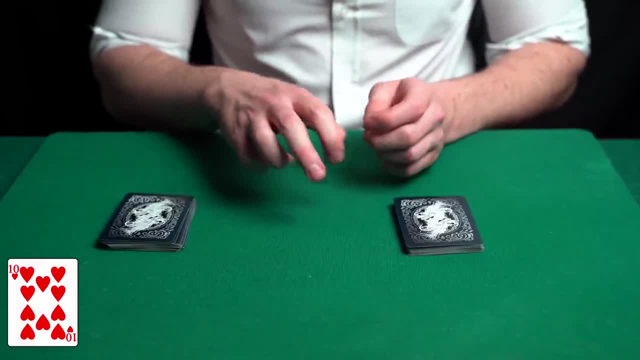 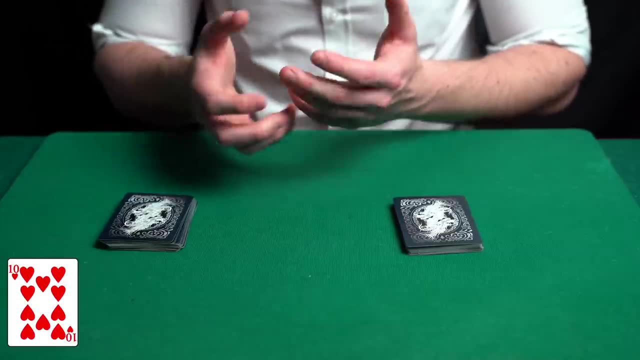 the spectator then cut the cards, chose what pile to use. then the spectator had a free choice to choose any card, which was then returned to the deck and shuffled. The magician then says he's going to show the spectator something impossible. He instructs the spectator to pick up the other. 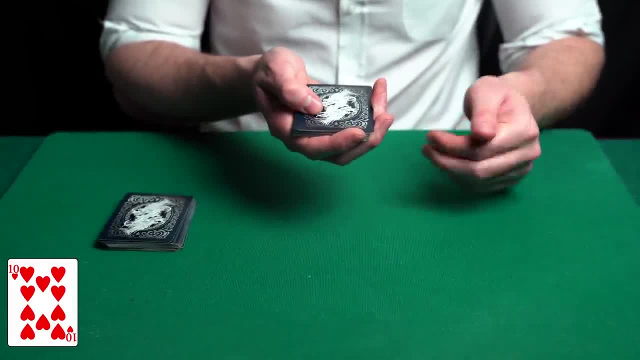 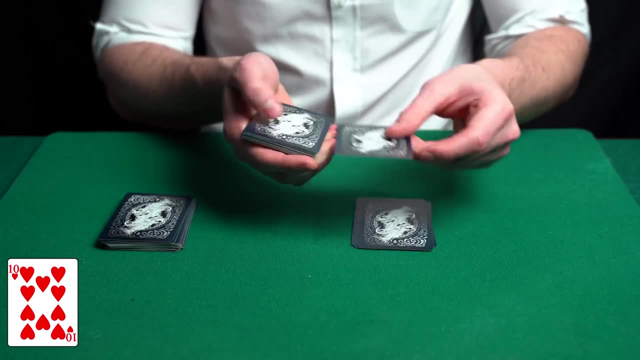 pile and deal the cards down and stop wherever they want. Wherever the spectator stops, the card that they choose will determine the location of the spectator's card in the other shuffled pack. The spectator stops and the magician then cuts the cards and chooses the card to lose the other pile. 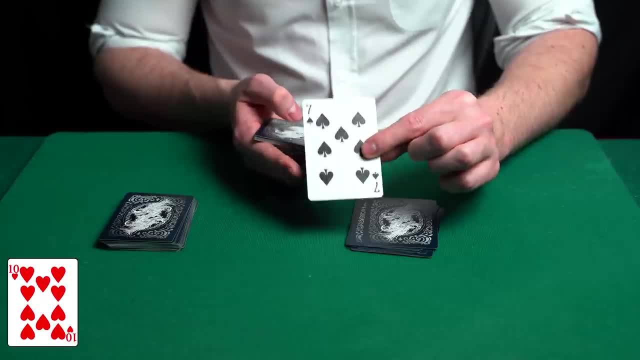 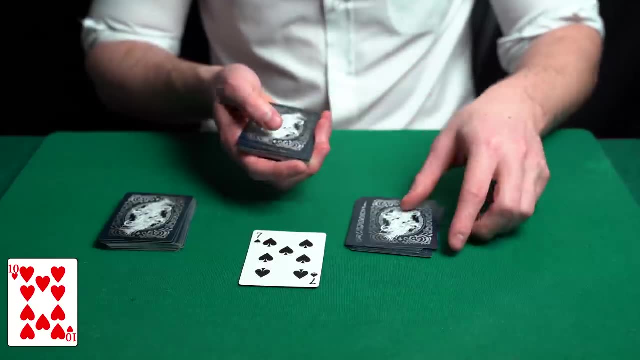 The magician tells them to turn their card over. It's a seven. Just to prove how random this was: had the spectator stopped one card later, it would have been a three, and one card earlier it would have been a nine. But they stopped at a seven And remember these cards were shuffled at the beginning of the trick. 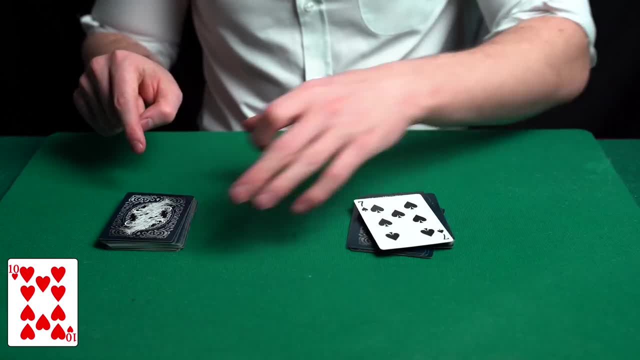 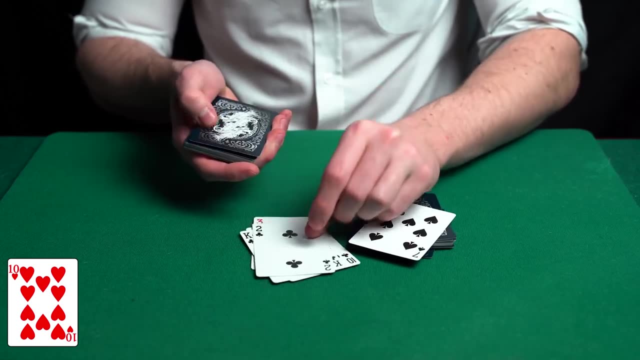 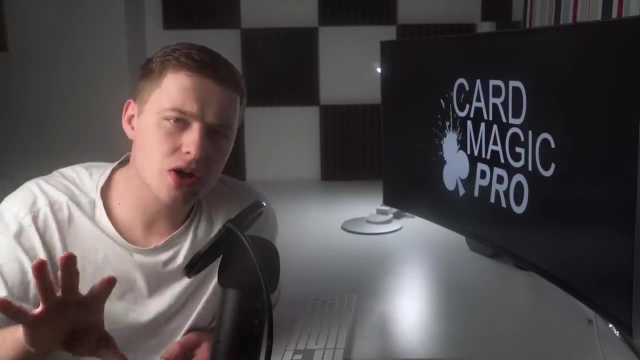 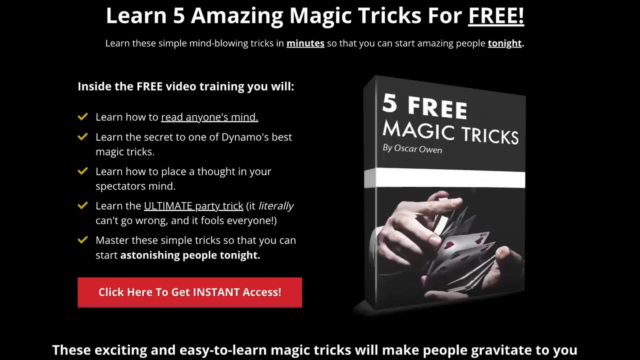 The spectator then picks up the other pack and counts off seven cards face up. The seventh card is their ten. The spectator is fooled Very quickly. if you want to learn five amazing magic tricks that are simply too good to reveal on YouTube, then sign up to my free magic masterclass. 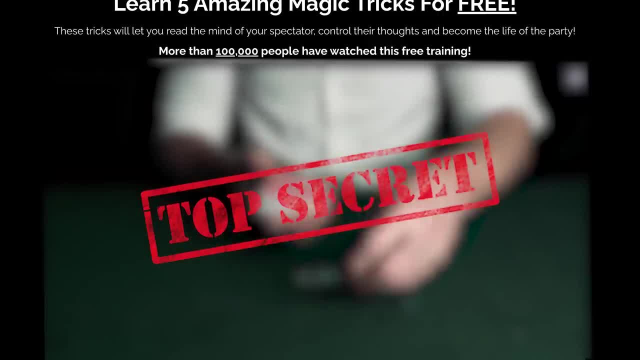 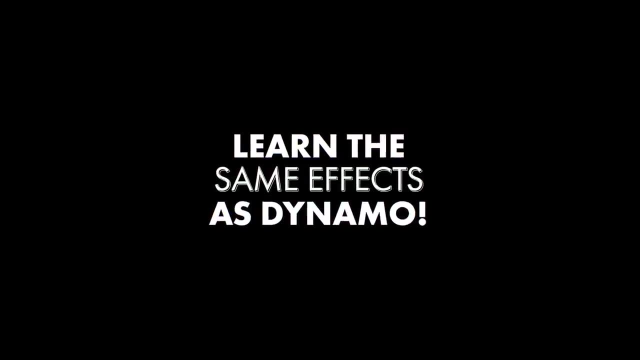 Inside the masterclass. I'm going to be showing you how to read the mind of your spectator. I'm going to be showing you how to put thoughts inside your spectator's head. I'll be teaching you the same effects that Dynamo uses when people tell him to perform. 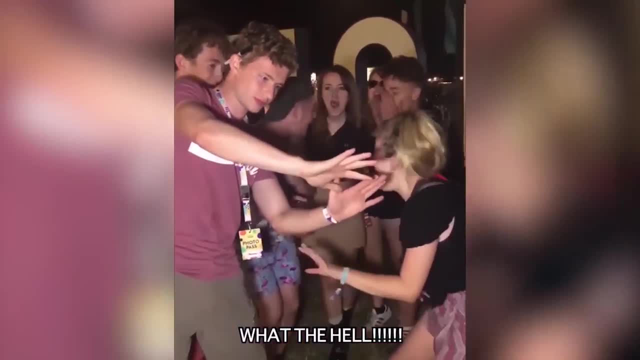 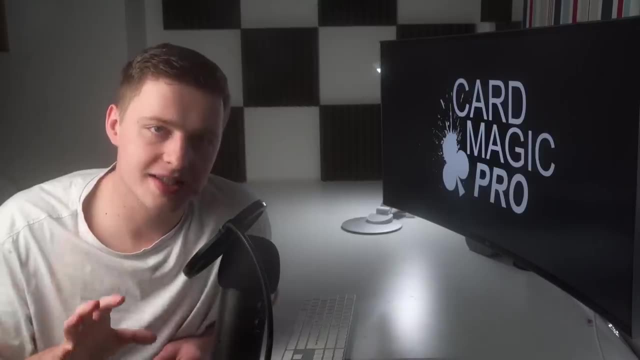 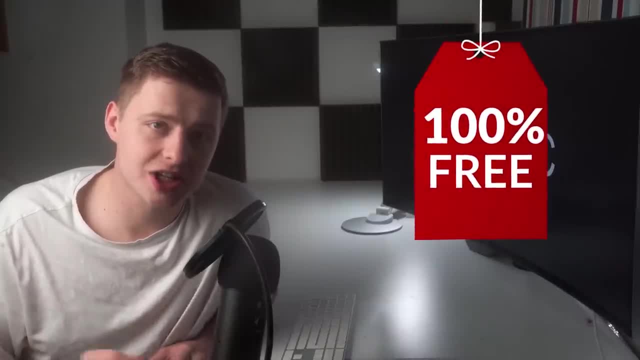 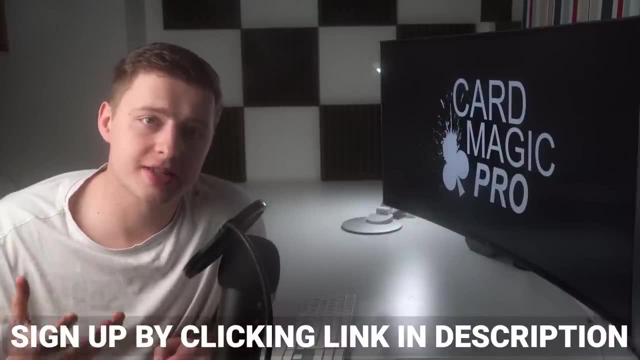 So the whole thing is 100% free. I really mean it. there's no strings attached. so just sign up by clicking the first link in the description and I'll teach you some mind-blowing magic tricks that you'll be able to perform within minutes of learning how to do them. 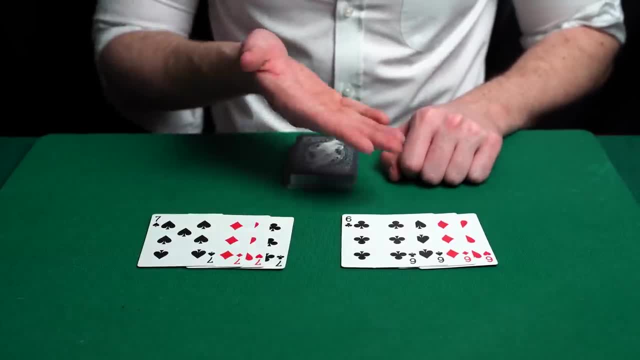 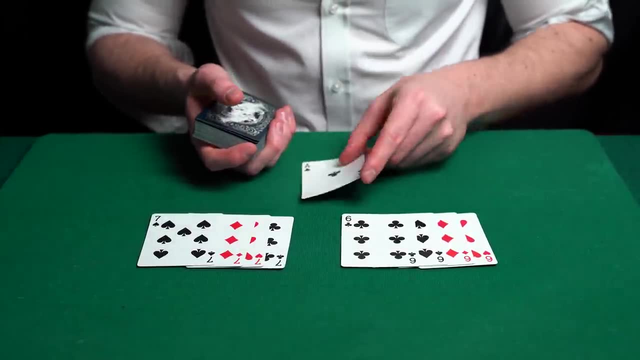 This trick requires a very simple setup and then from there it's basically self-working. Remove all the sixes and sevens from the deck and then do the following: Place one random card onto the deck, then place a six, then place another random card onto the deck. 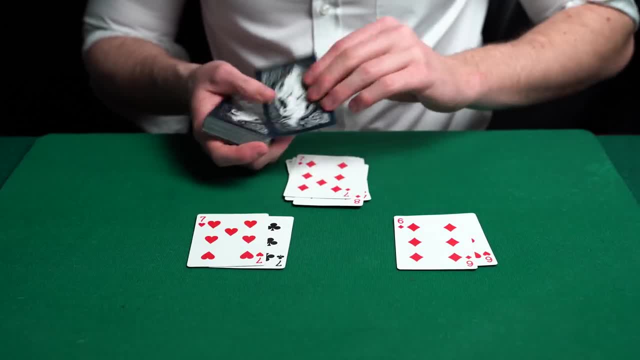 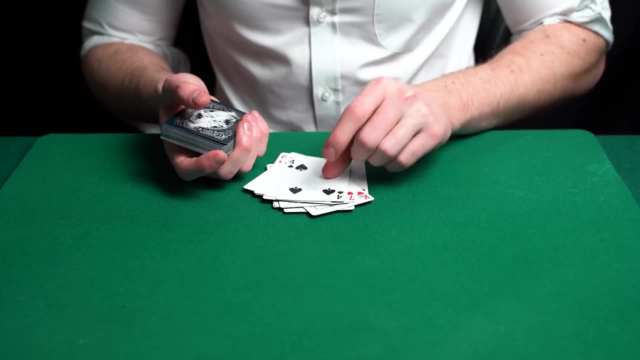 then place a seven and keep doing this until all the sixes and sevens are used up. It doesn't actually matter what order you place the sixes and sevens in, so long as there's a random card in between them Very quickly. a more advanced way of doing this, as I did in the performance. 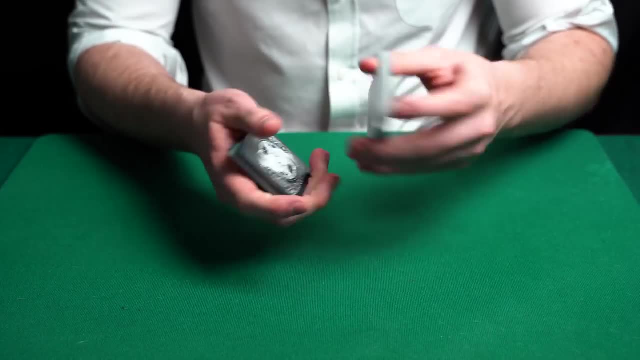 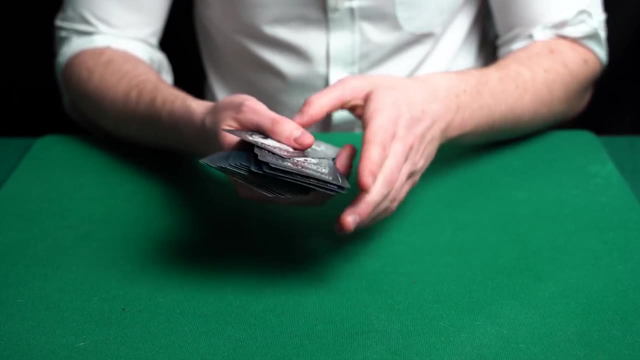 is to place all the sixes and sevens on top of the deck, Then begin by doing a perfect faro shuffle and all the cards will interlace. as you can see, The cards will now be in a stack. However, if you don't know how to do a faro shuffle, then don't worry. 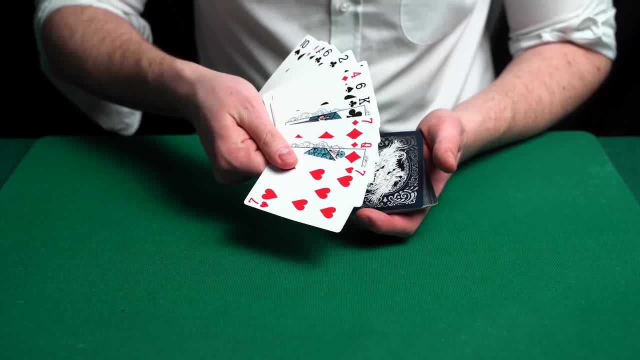 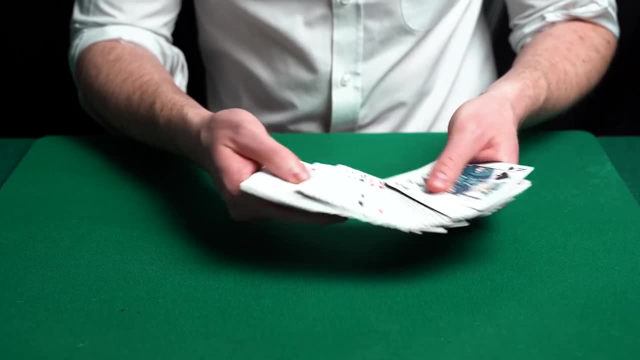 just begin by stacking the cards, as I've just showed you. So now, regardless what method you used, you should have a stack on top of the deck. You can actually spread out the cards to show that they're completely normal, and as the stack is basically impossible to see, 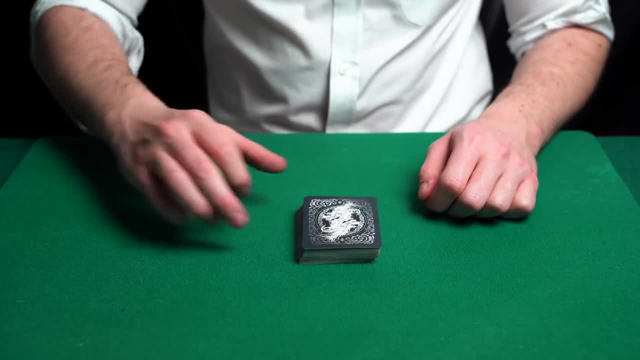 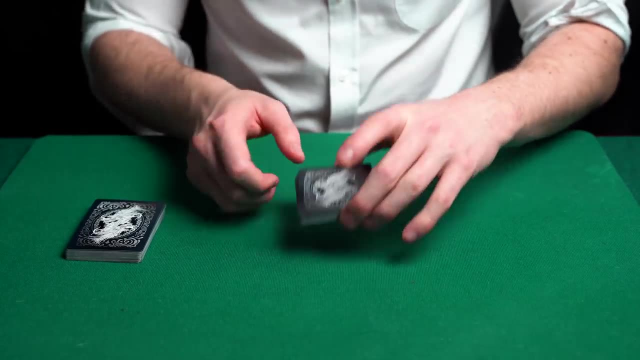 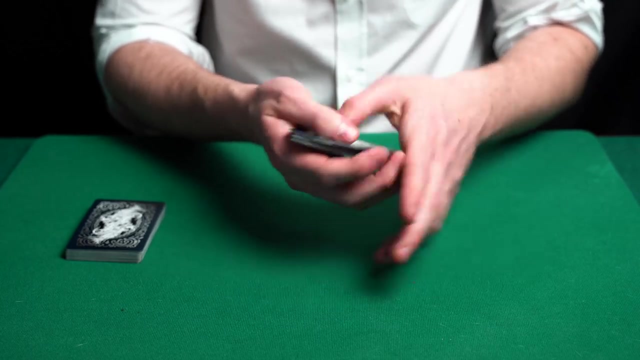 Ask the spectator to cut the cards in half. Take what was the top half of the deck and place that to the side. Then take the other pile and shuffle them in any way you like. Now let the spectator choose any card. However, as you do this, count off the top six cards. 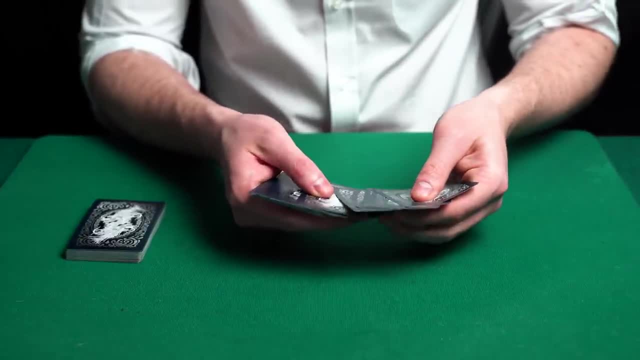 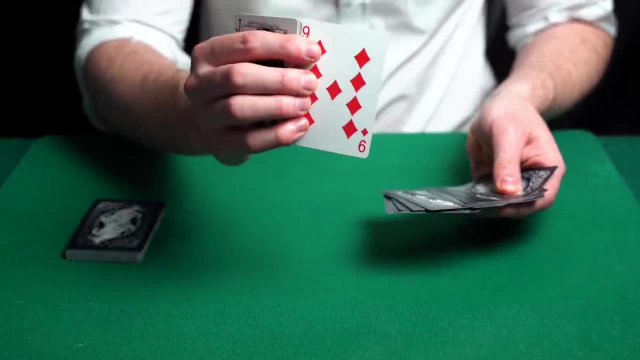 by pushing them to the side and then place your fingers under them. So in your hand you're holding the top six cards. Now let your spectator pick out any card- In this case they've chosen the nine of diamonds- And when they return that card, just place those other six cards on top of it. 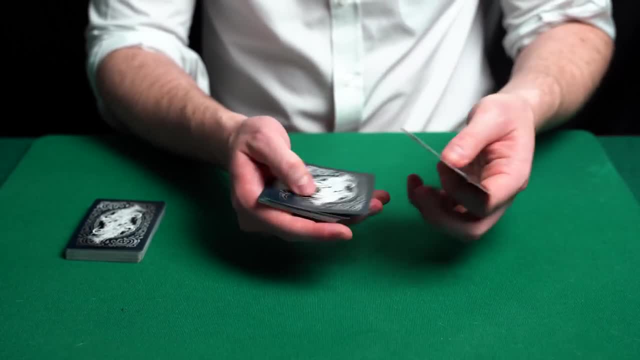 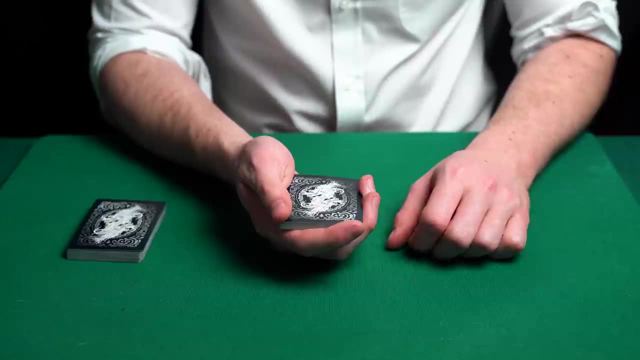 This will place their card seventh from the top. If they happen to choose a card from the six cards that were in your hand when you were spreading them out, then very simply just add an extra card into the stack whilst they're looking at their card. 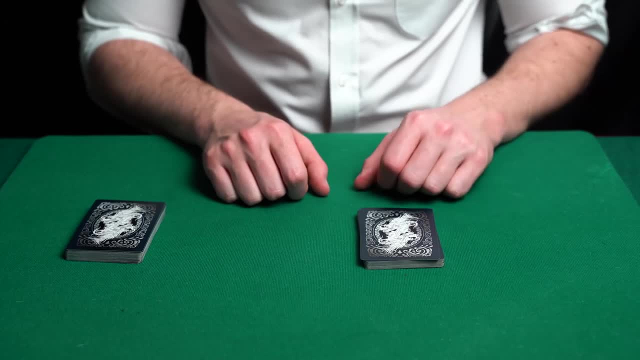 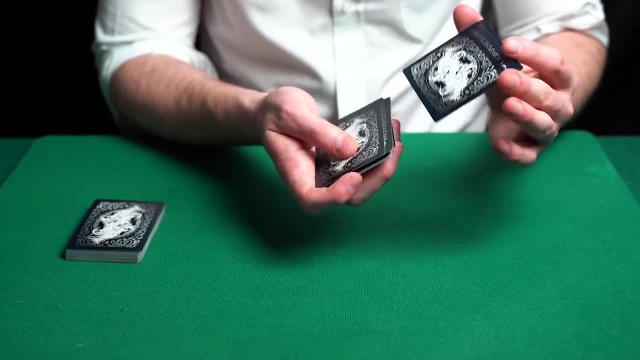 You've got all the time and misdirection in the world to do this. So you place their card back into the deck, drop it onto the table and act like nothing has happened. They chose a card, they put it back and that was that. 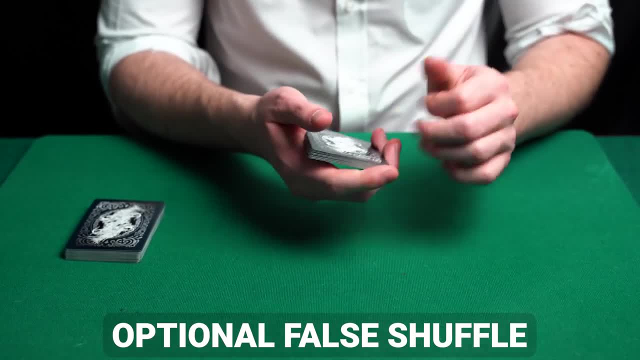 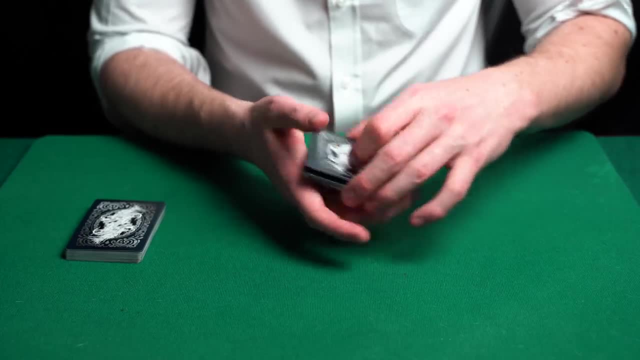 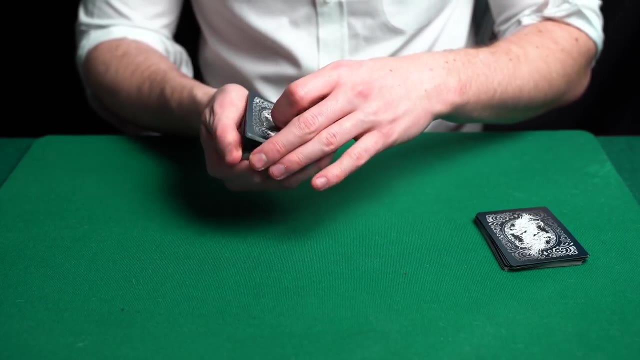 If you want, you can perform a false overhand shuffle like I did in the performance, but again, this is really not needed. Now let the spectator pick up the card the other pile and tell them to deal down and say: wherever you stop at, that card will determine the location of your selection. 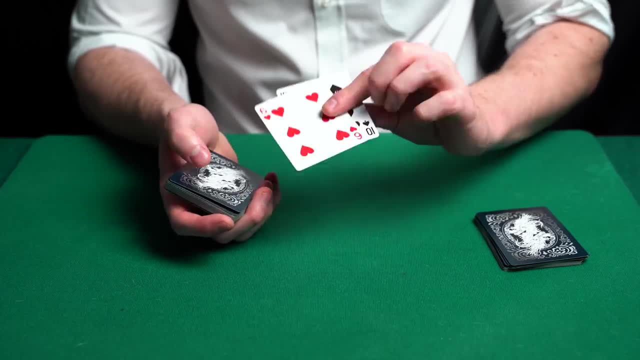 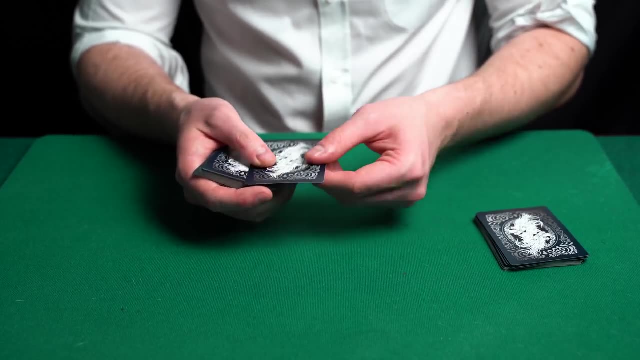 Remember that every other card is a six or a seven. So you have a random card, then a six or a seven, then a random card, then a six or a seven, and so on. So let the spectator deal down. and when they deal to a random card, think no.